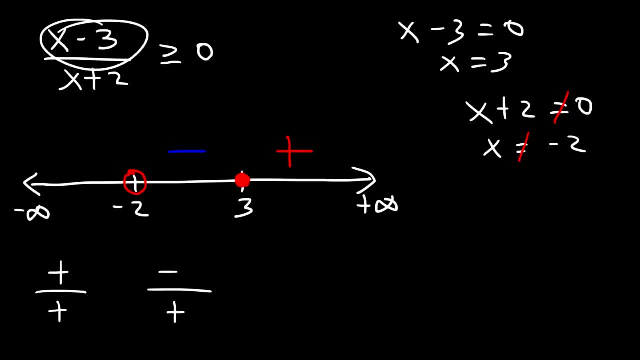 region like negative 3.. Negative 3 minus 3, that's negative 6, so that's negative. Negative 3 plus 2 is negative, And two negative numbers divided against each other will produce a positive result. Now we want the fraction to be greater than or equal to 0. So we want the 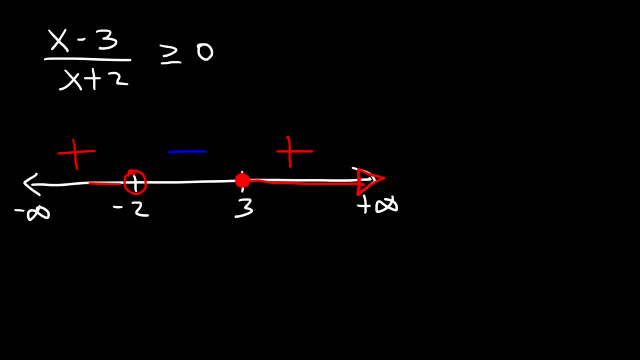 positive values. So we're going to shade that region and the region on the left. So the solution in interval notation is going to be negative infinity to negative 2 with parentheses due to the open circle, And then union 3 to infinity using brackets due to the closed circle that we 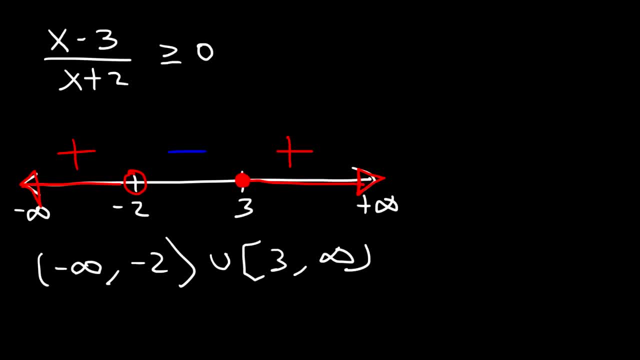 have here Now to express the same answer using inequalities. for this part, you could say that x is less than a negative 2, or for this part, x is equal to or greater than 3.. So those are the two ways in which you can express your answer. So 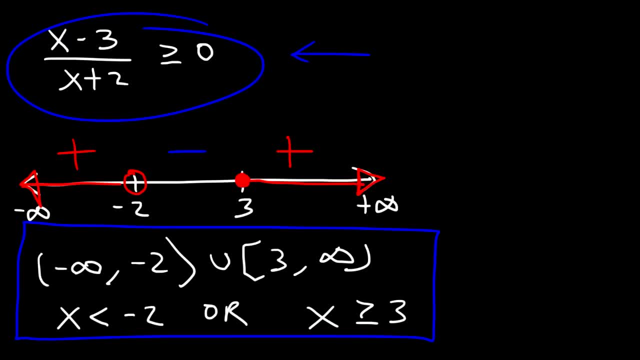 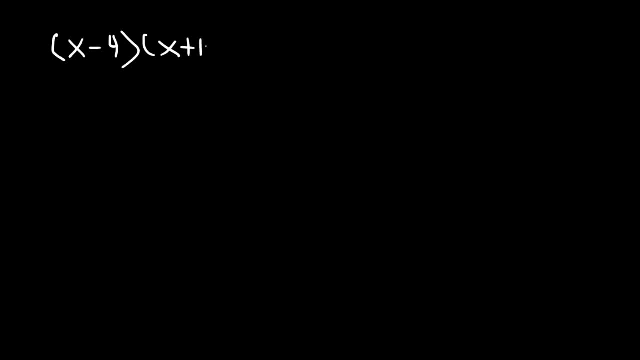 that's how you can solve this particular rational equation: Inequality. Let's try another example: x minus 4 times x plus 1 divided by x minus 3. And this is going to be less than 0.. Feel free to pause the video if you want. 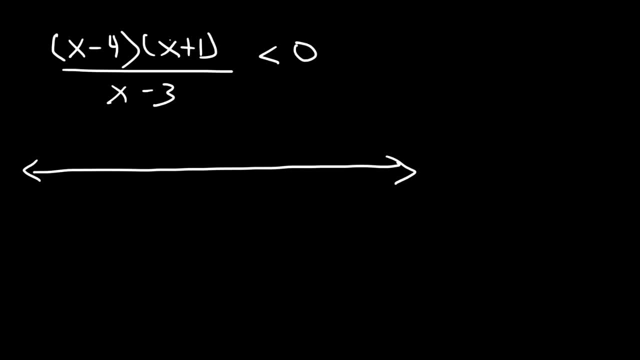 to. So the points of interest are negative: 1 and then 3, and then the next one is 4.. We're going to have positive infinity and negative infinity. Now this one is in a denominator, so we're going to have an open circle at 3.. Now notice that it. 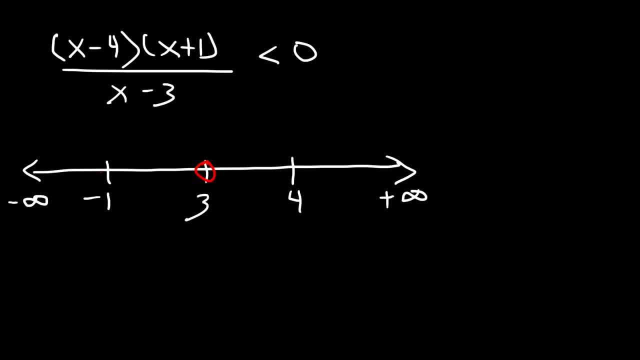 doesn't equal 0. It's less than 0. So, in fact, all of these points of interest will be open circle. If it was less than or equal to 0, these two would be a closed circle. So keep that in mind. 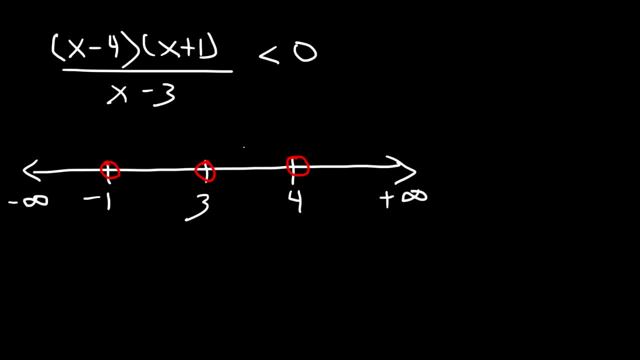 Now, because it's less than 0, we want to find the regions that are negative and not positive. So let's check the signs. Let's pick a number between 4 and infinity, Let's use 5.. So 5 minus 4, that's going to be positive, And 5 plus 1 is positive 5. 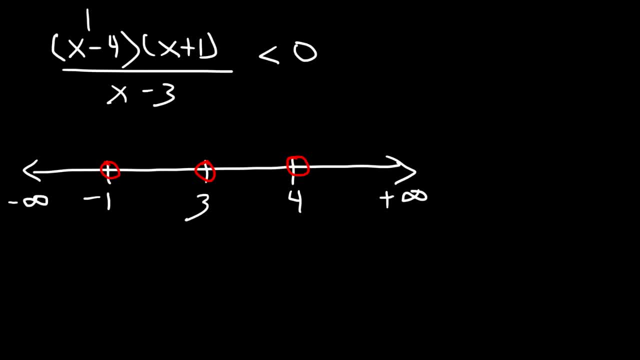 minus 3 is positive, So the first result will be positive. Now, if we pick a number between 3 and 4, like 3.5, 3.5 minus 4 is negative, 3.5 plus 1 is positive and 3.5 minus 3 is positive. So a negative times a. 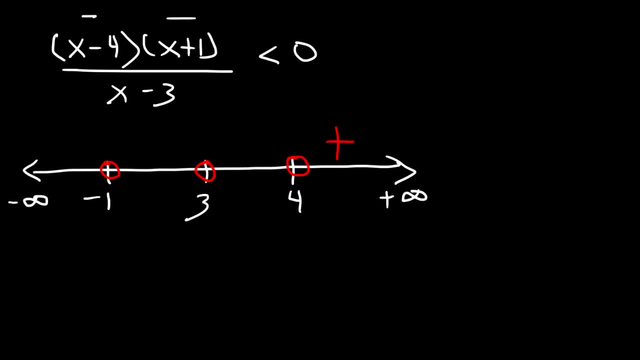 positive times. a positive will give us a negative number. Now, picking a number between negative 1 and 3, let's try 0.. 0 minus 4 is negative. 0 plus 1 is positive. 0 minus 3 is negative. 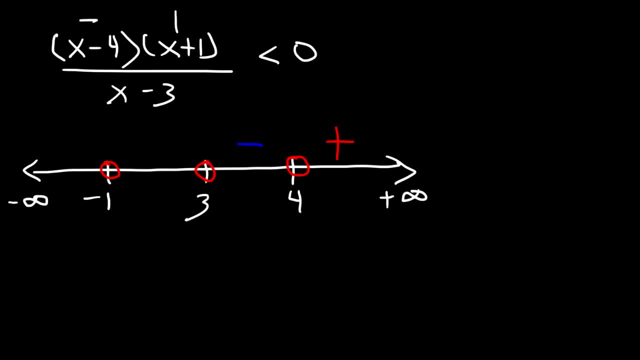 A negative times, a positive times. a negative will give us a positive number. Now, the signs will always alternate if the multiplicity of each 0 is 1. So the next one is going to be negative. If you plug in negative 2,, this will be negative. 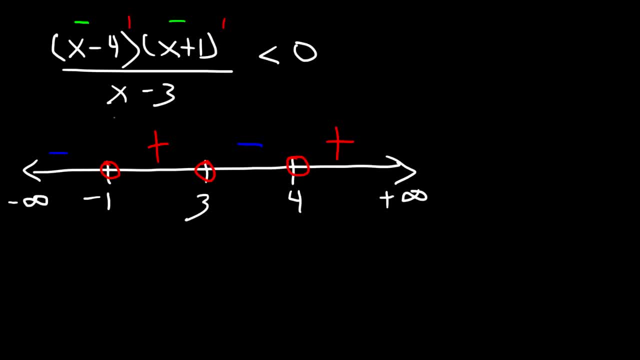 Negative: 2 minus 4 is negative. Negative 2 plus 1 is negative. Negative 2 minus 3 is negative. Three negatives multiplied to each other will be negative. Now we want the portion of the graph that is less than 0, or that's negative. So the answer: 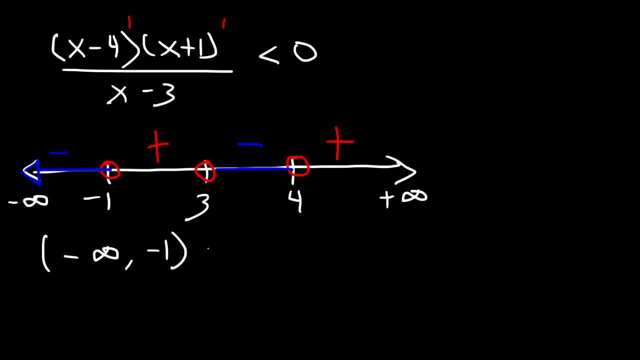 using interval notation is going to be negative. infinity to negative 1, union 3 to 4.. As an inequality, we could say that x is less than negative 1, or x is between 4,, between 3 and 4.. And that's it for this problem. Let's work on this one. 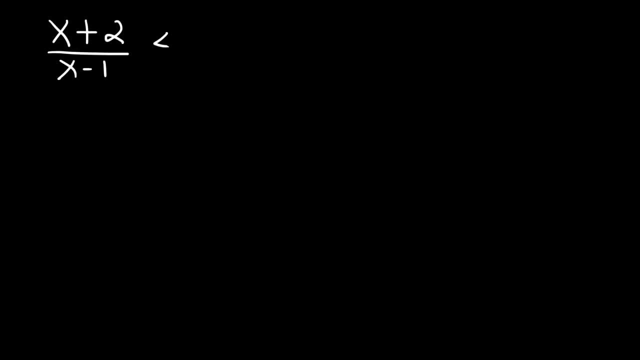 So x plus 2 over x minus 1, let's say it's less than or equal to 3.. So what do you think we need to do in this case? Because this is not 0. So we need to do some work before we. 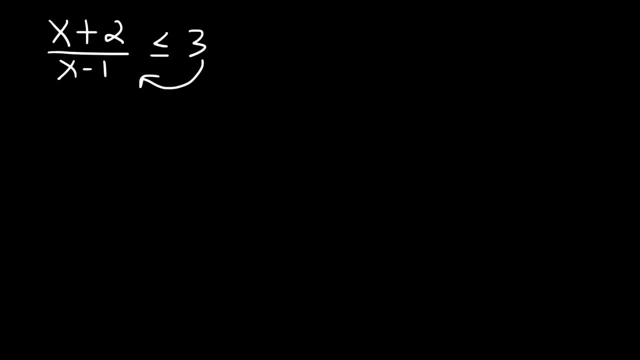 can make a number line. Let's move the 3 to the other side, So it's going to be x plus 2 over x minus 1 minus 3. And so that's less than or equal to 0.. What we need to do at this point is multiply negative 3 by x minus 1 over x minus 1.. We 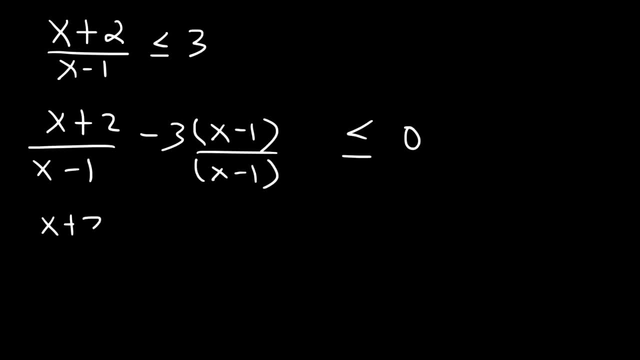 need to get common denominators. So this is going to be x plus 2 minus 3 times x minus 1.. And because the denominators are the same, we can write it as one single fraction. So now let's distribute the negative 3 to x minus 1.. So it's going to be negative 3. 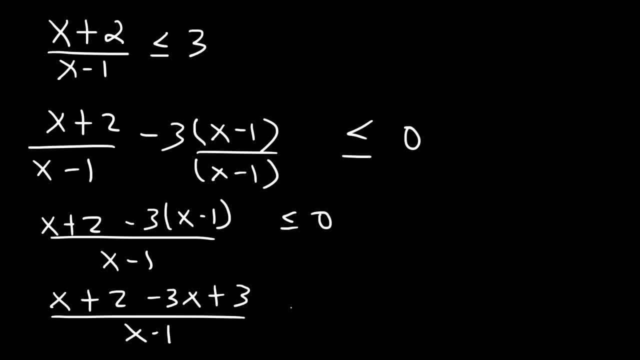 x plus 3.. And now let's simplify. So x minus 3 x is negative, 2 x And 2 plus 3 is 5.. So this is what we now have. Now we know that the denominator cannot be 0. So therefore, x can't be 1.. And if we set 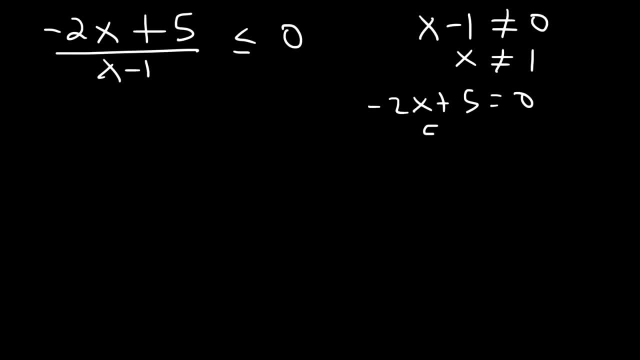 the numerator equal to 0, then 5 is equal to 2 x. So x is 5 over 2, or we could say 2.5.. So those are the points of interest. So we have 1 and 2.5.. Now we're going to have a closed circle at 2.5 and an open circle. 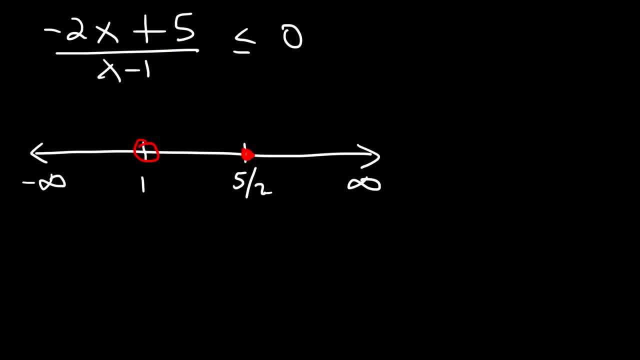 at 1, because you can't have a 0 in the bottom. Now let's test the points. So let's try a number that's bigger than 2.5.. Let's try 3.. So negative 2 times 3 plus 5 over 3.. And 2 is equal to 3.. And this is our derivative, So we just write it as negative: 1 x 3 plus 5.. So let's try a number that's bigger than 2.5.. Let's try 3.. So let's try 3.. So negative. 2 times 3 plus 5 over 3.. Now let's see what this is equal to. Let's put the whole number together, So we have negative 2 times 3 times x minus 1 plus 5 over x minus 1.. And just get the. 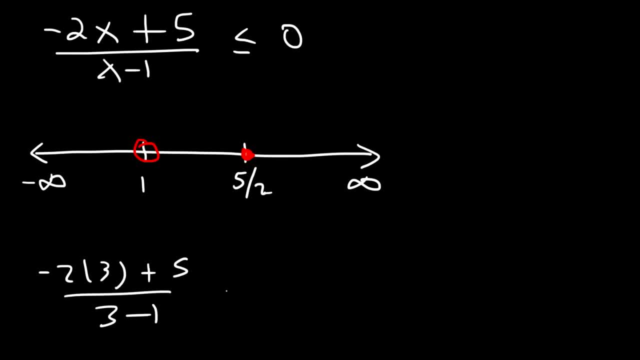 Over 3 minus 1. negative 2 times 3 is 6. I mean negative 6 plus 5. That's negative and 3 minus 1 is positive. So here we have a negative result in this region and if we pick a number between 1 and 2.5, like 2,